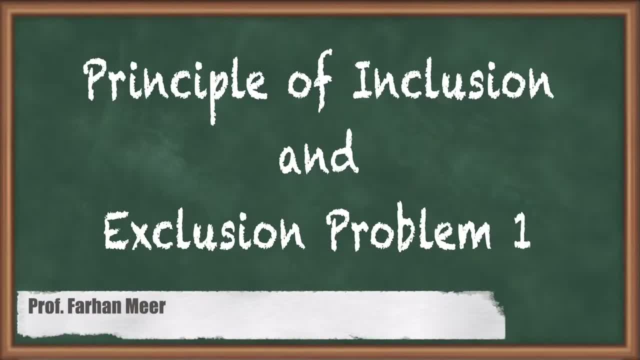 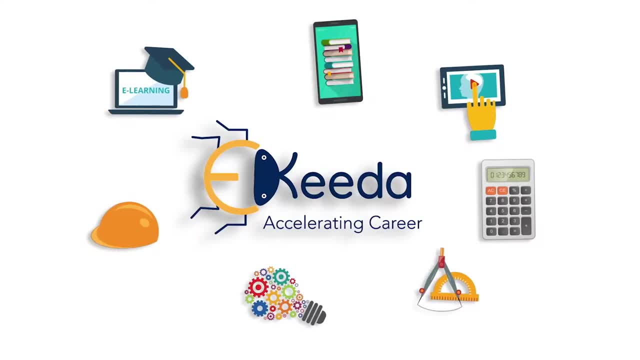 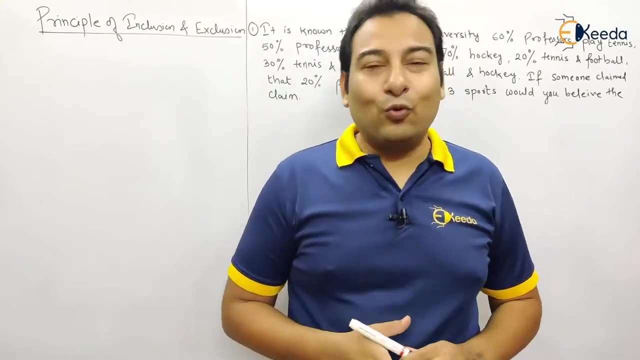 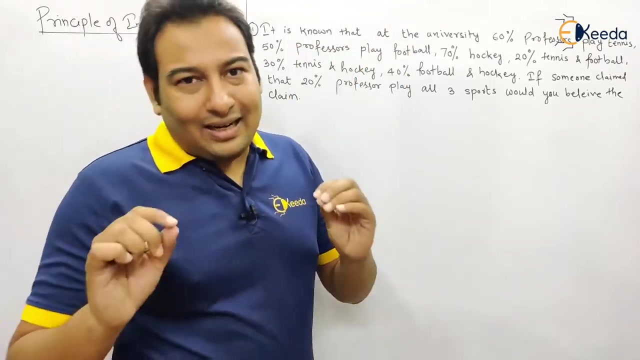 Hello friends, in this video we'll be discussing principle of inclusion and exclusion, problem number one. Welcome back, friends. Now we're starting with the new topic- principle of inclusion and exclusion, also called counting principle- and it's very simple principle, So let us understand first. 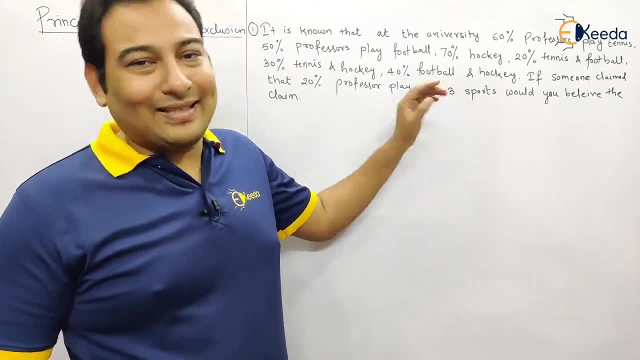 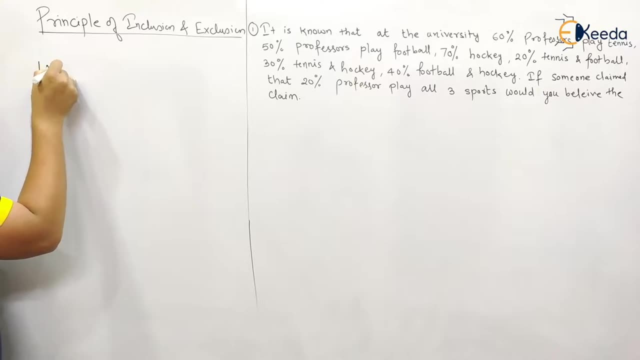 what is the principle? and in the same video we'll be solving one example on the same principle. So let us start See. suppose there are two elements. This is called cardinality. Cardinality means number of elements, So A union, B. 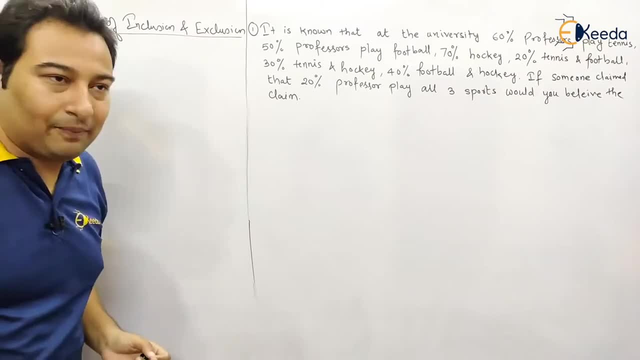 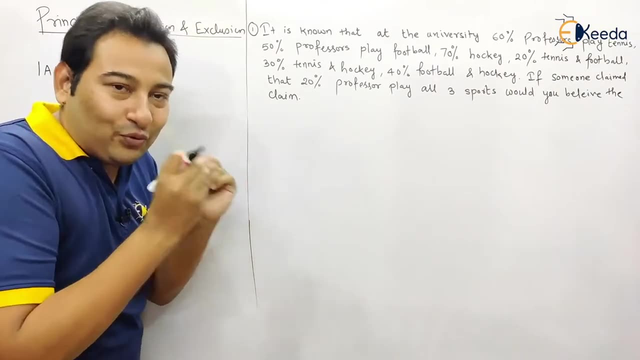 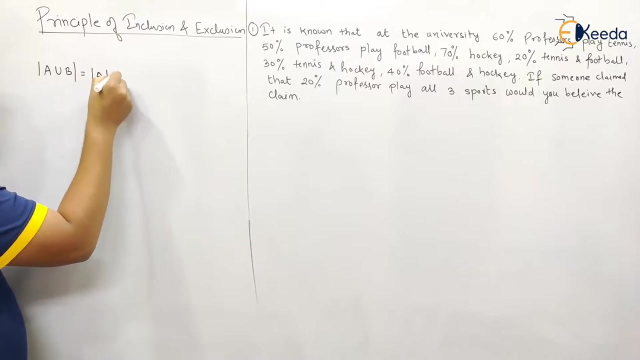 this indicates number of elements in A union B. So that is equal to: we are going to include few things and we are going to exclude few things. So all the single elements will be included first. So what are the single elements here? A and B. So A and B, single included, double excluded A, intersection B. You need to remember. 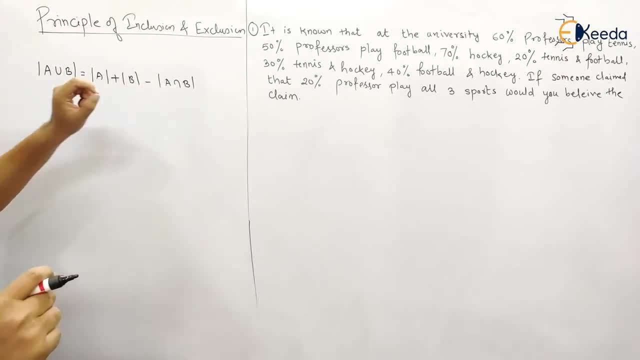 on left hand side, it will be union, on right hand side it will be intersection. So this is the formula: if there are only two terms or two elements, All single included, double excluded. And what does this cardinality mean? It indicates: 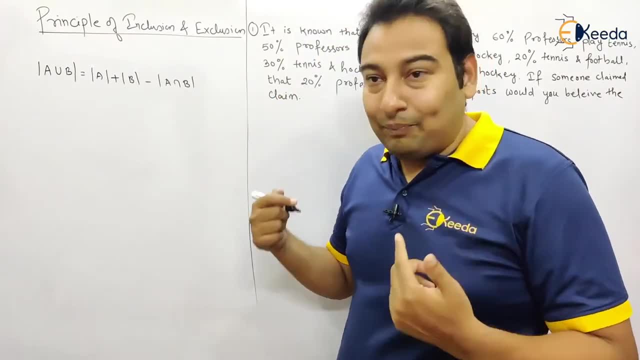 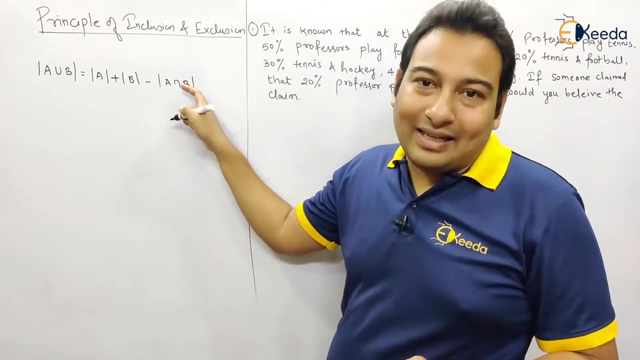 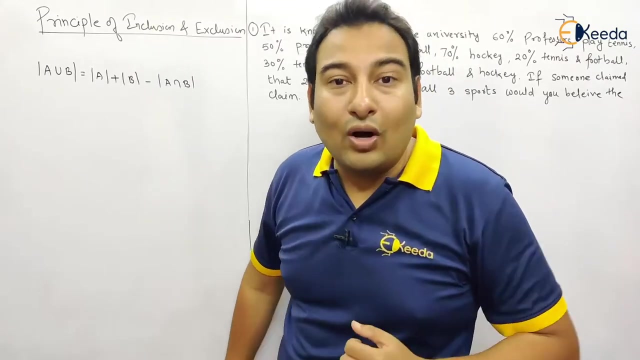 the number of elements. We are not going to understand from this what are the different elements in A intersection B? We'll just get to know how many elements are there. For example, if there are 60 students in a class, so this will indicate 60. We will not get to know who are the different students. 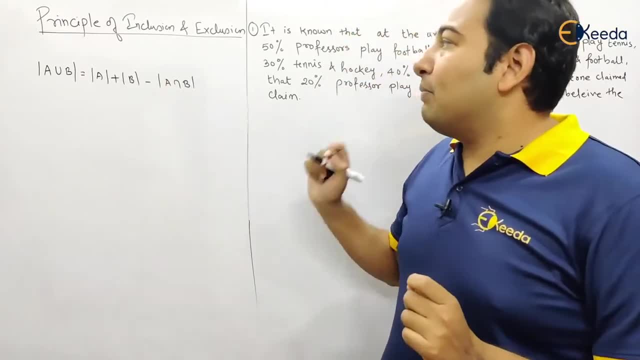 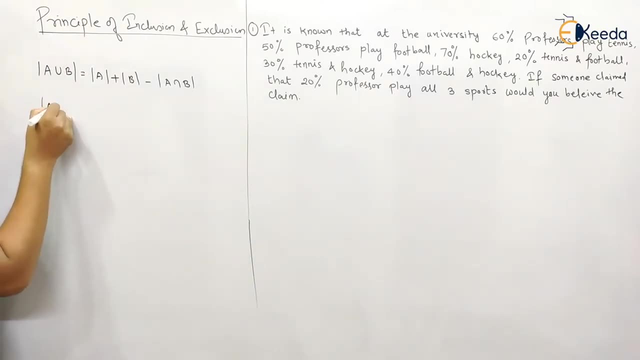 Are you clear with this? This indicates number of elements. So this is principle of inclusion and exclusion for two elements. Generally in the exam we get problem of three elements. So we will design a single number and we'll come to definition by defining 3 elements. 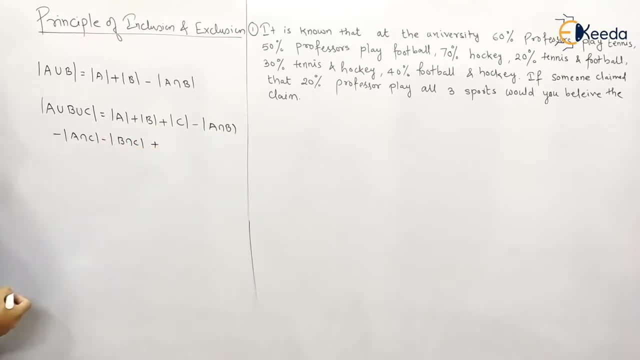 Explain this With reference. you just understand the data, Are you sure? Yes, OK, Let me read these out: plus alternate, plus minus, single included, double excluded, triple included. so what are the triple terms? a, intersection b, intersection c. so this is the formula, if there are three elements. now 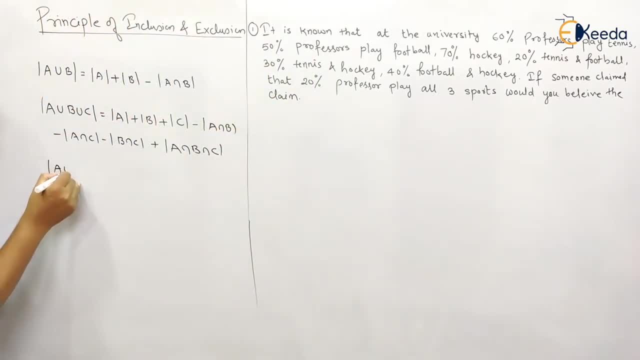 we'll discuss formula for four elements. generally you can say 80, 90 percent of the times this formula is used in the exam. now there will be four items. what is the formula? the concept will remain same. all the single terms will be included. that means a plus b plus c plus d, all the single. 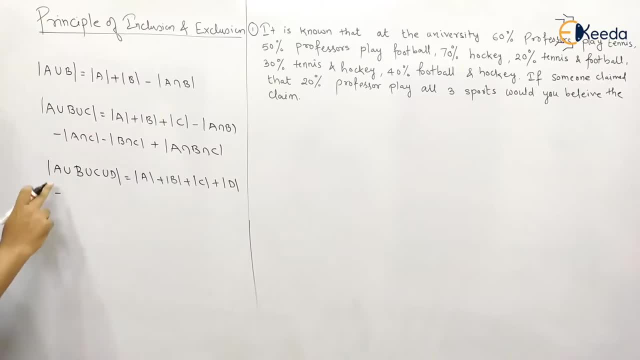 term included all the double term excluded. what are the different double terms? a, b, a, c, a d. first we'll start with respect to a, so a, b, a, c, a d, then with respect to b, b, c, b d and finally c: d. a, b, a c. 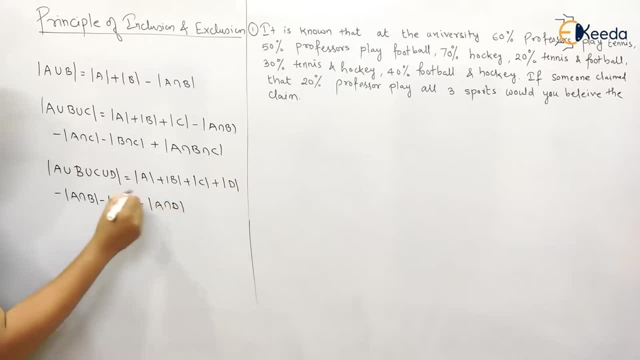 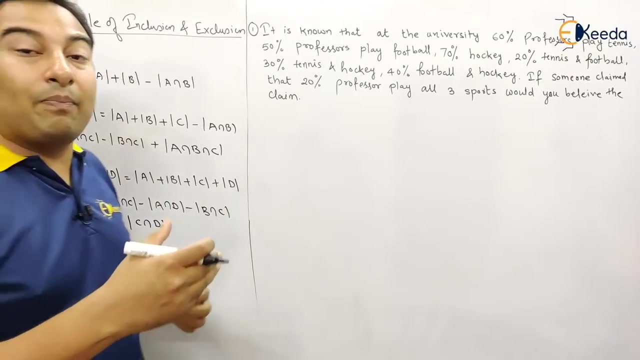 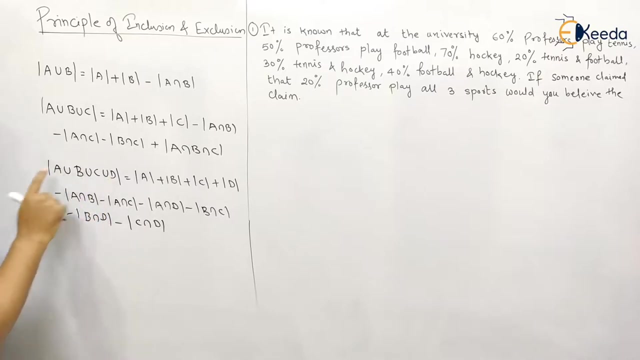 b is alternate plus minus single term, plus double term, minus triple term, plus a b c, next a b d, next a c d and finally b c d. you check with the combination. there are only three possible combinations and four different combination possible with respect to three terms. so single included. triple included. double excluded. double included. four excluded a. 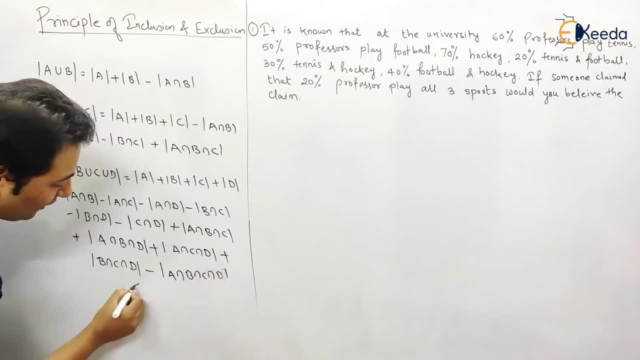 intersection b, intersection c, intersection d and so on. so this formula can be extended to n terms. so we have a formula for 5 terms, 6 terms and so on. but generally you can say 80 percent times or 90 percent time. this formula is useful generally. example are given on three elements. up: 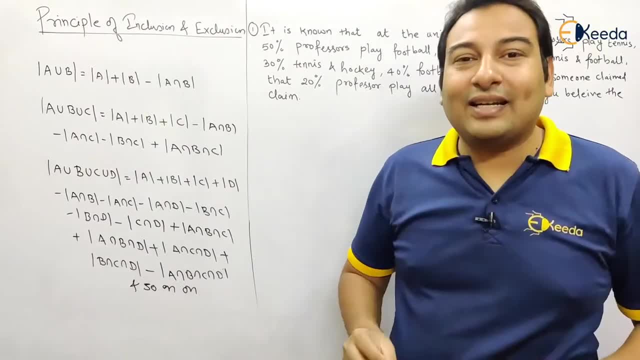 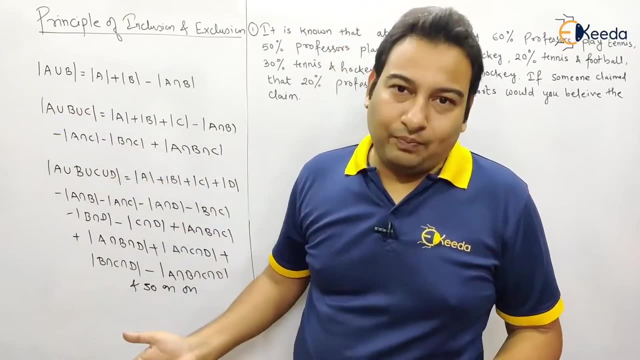 to r sub sok in imperial and t ext比如 five and r sub c, like a egg in balachanish pushing r subussy in pprofessionalian r sub, cylinder r sub hottest sound and large r sub. I hope the formula is clear. Now we will discuss one example on the same formula. 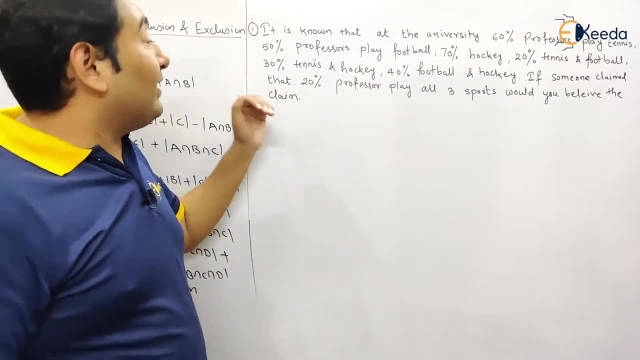 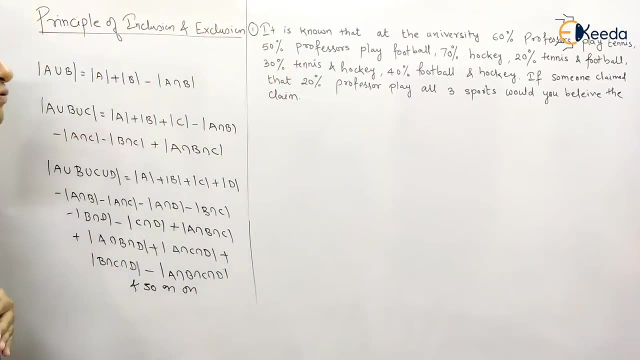 Let us read the question first. It is known that at the university 60% professor play tennis, 50% professor play football, 70% hockey, 20% tennis and football, 30% tennis and hockey, 40% football and hockey. 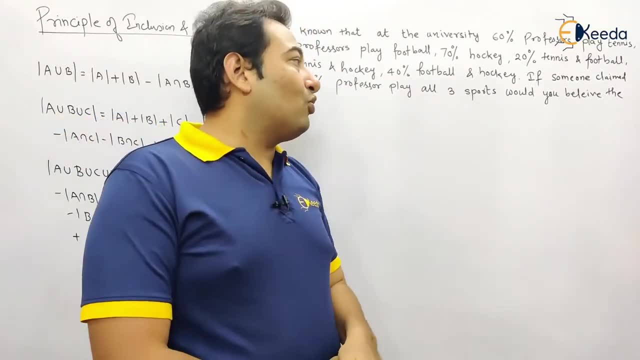 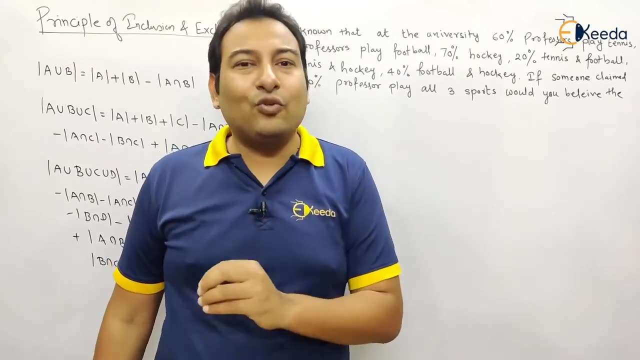 If someone claimed that 20% professor play all the three sports, would you believe the claim? The question is: there are few professors- X number of professors in the university. Some play football, some play tennis, some play hockey, some play both and so on. 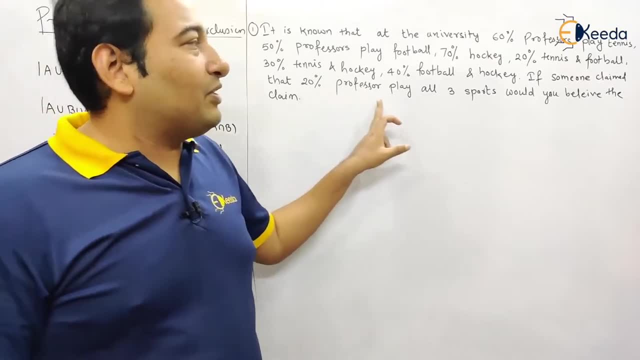 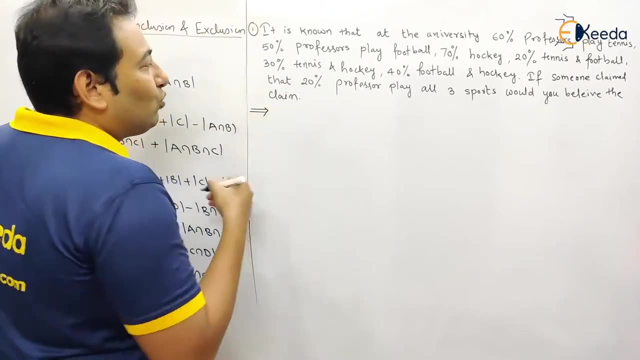 And we need to check. there is a claim: 20% professor play all the three sports. We need to check whether the claim is right or wrong. So let us start. First of all, we need to assume how many professors are there. 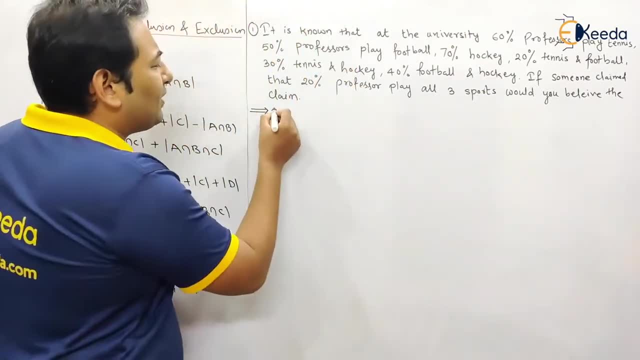 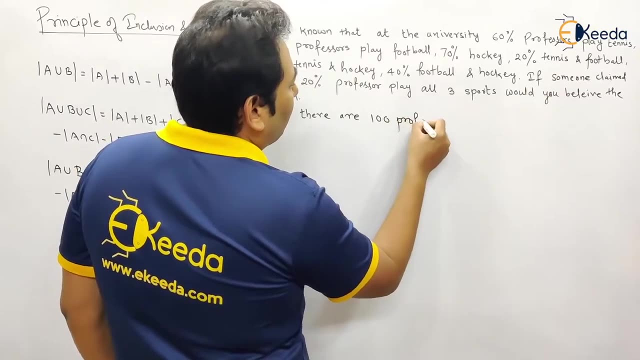 See, nothing is mentioned. how many professors are there? So let me assume let there are 100.. Why we are assuming 100 professors? Because all the terms are given in percentage. So if there are 100 professors you can easily calculate. 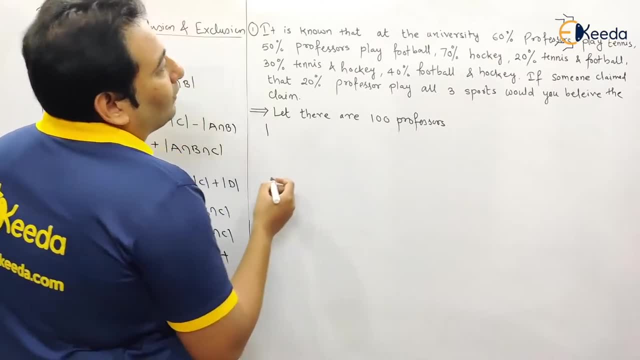 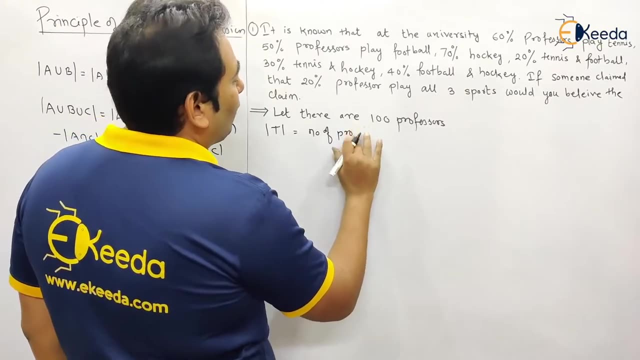 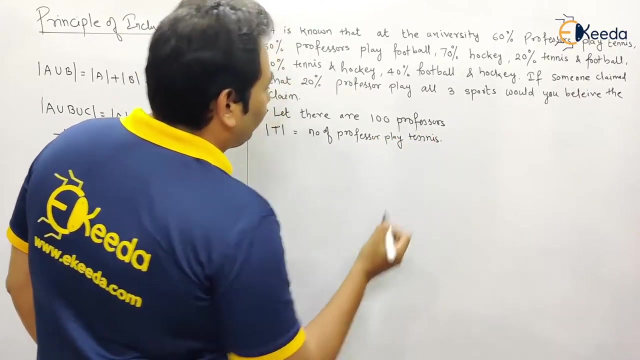 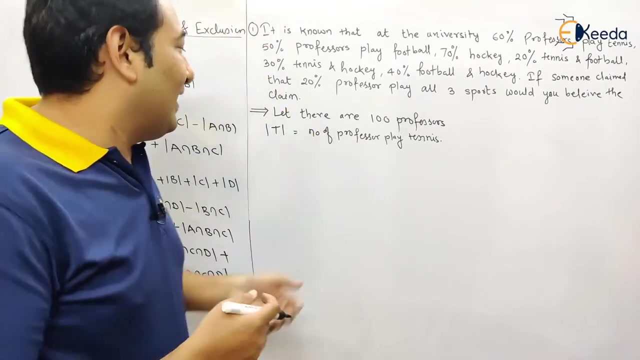 Let us say mod t, number of professors play tennis. Let us assume This is your cardinality. So let me assume mod t denotes the number of professors play tennis. And the same way, mod f is equal to number of professors play football. 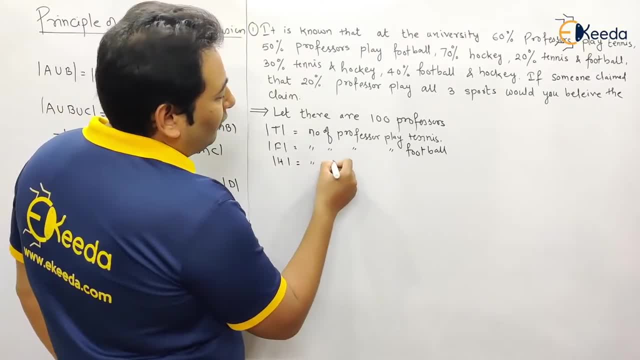 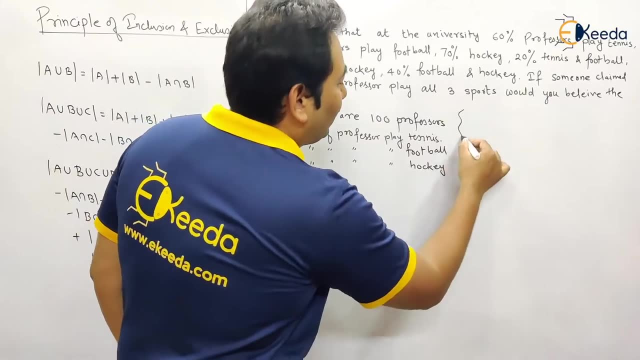 And there is last term, hockey. So let us say mod h number of professors play hockey. Now let us read the data and let us try to analyze what are the different things given in the problem. See, I do not have that much space. 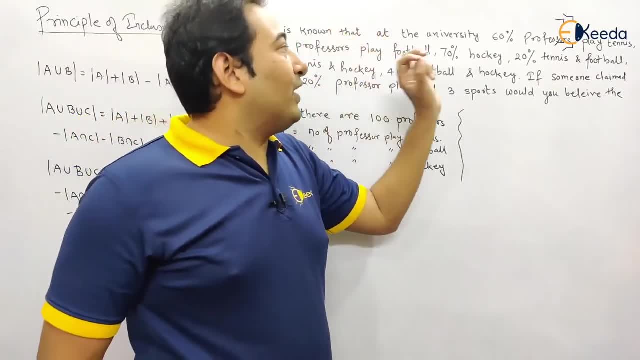 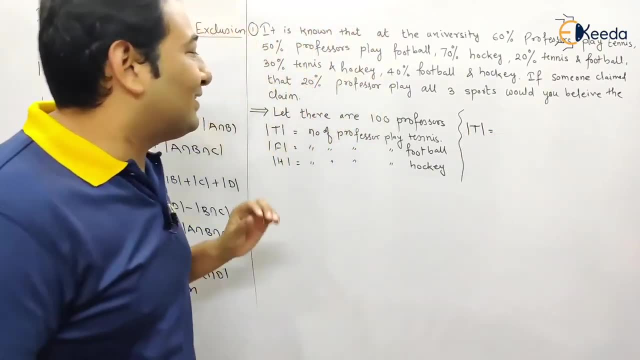 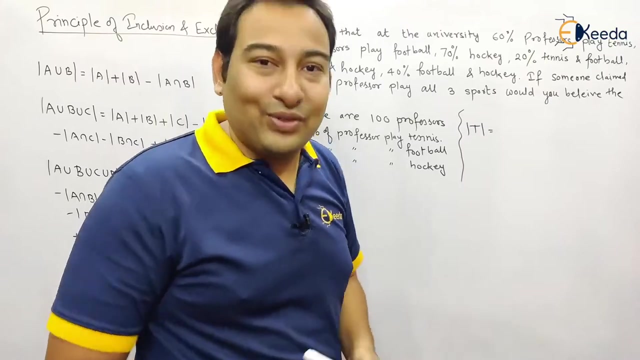 Therefore I am writing down here. So what is the first? The first thing, given it is known that at the university, 60% professor play tennis, So mod t will be what 60% professor? Since there are 100 professors, 60% will become 60.. 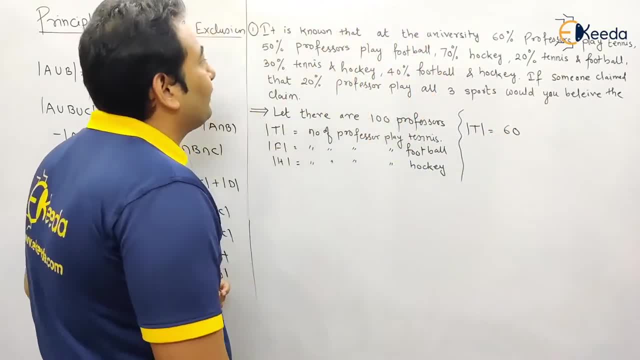 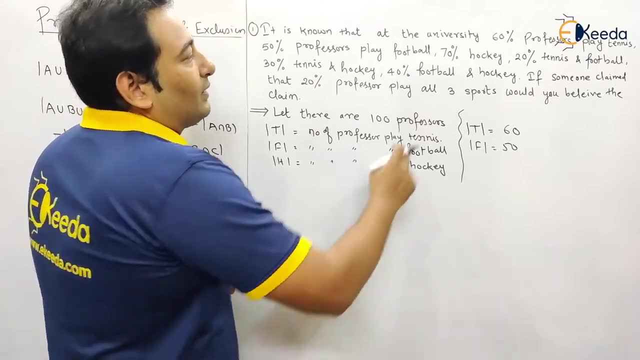 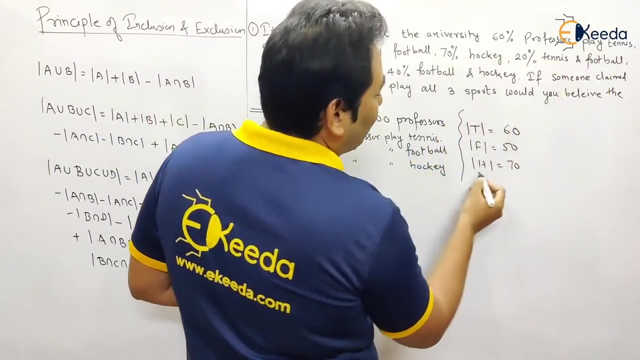 So there are 60 professors which play tennis. Next 50% professor play football. So football will be 50%, 70% hockey. So hockey is 70%. What is next? 20% tennis and football. 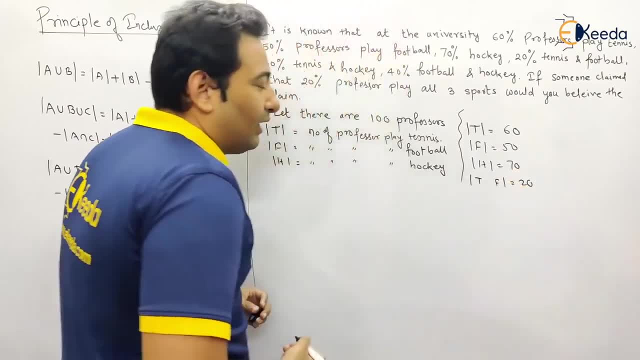 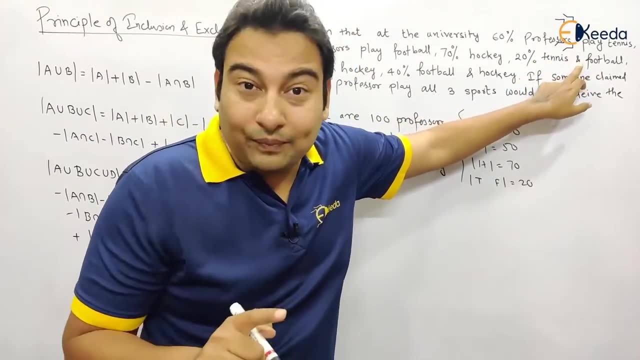 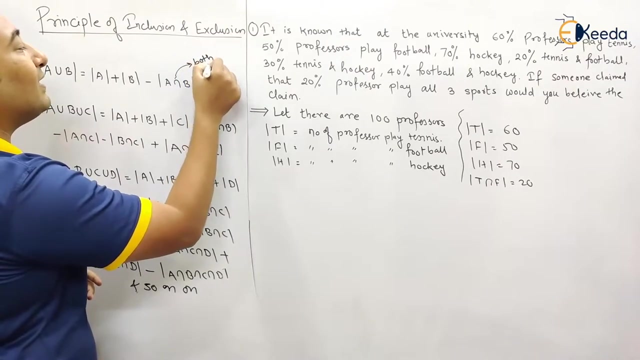 Tennis and football is what 20.. Now, please tell me, it is and Tennis and football. So what do you mean by and? And means both. That means it is intersection If you get both, or and basically. So this is intersection. 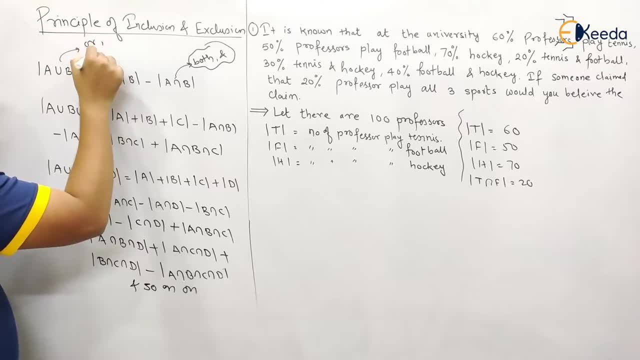 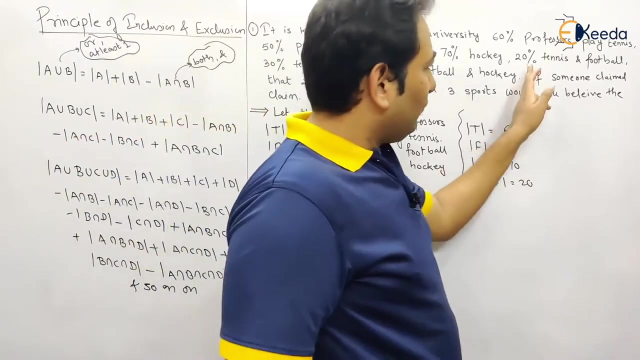 And, Or at least one, something like this, then it is union and means both, or means and means intersection, or means union. So here it is given: 20% played tennis and football. So tennis and football is 20%, What else? 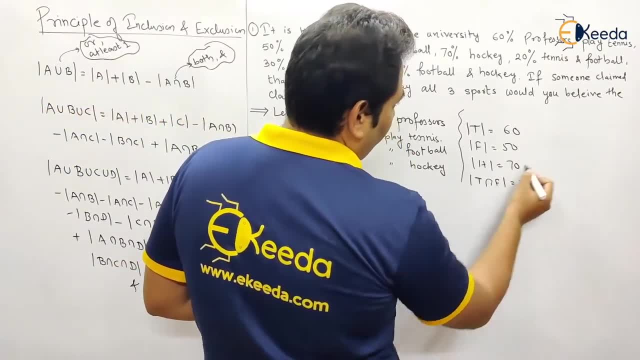 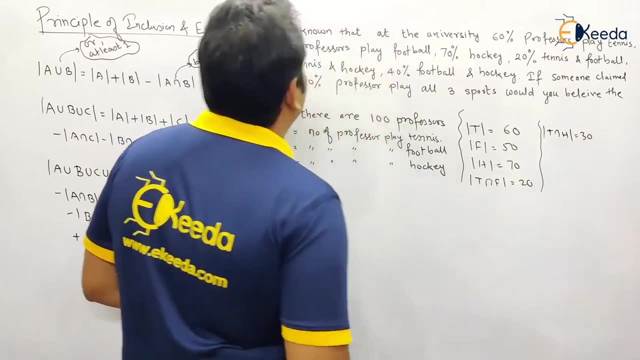 30% tennis and hockey. So what else? 30% tennis and hockey. So what else? 30% tennis and hockey. So what else? Tennis and hockey is 30%. What else 40%? football and hockey? 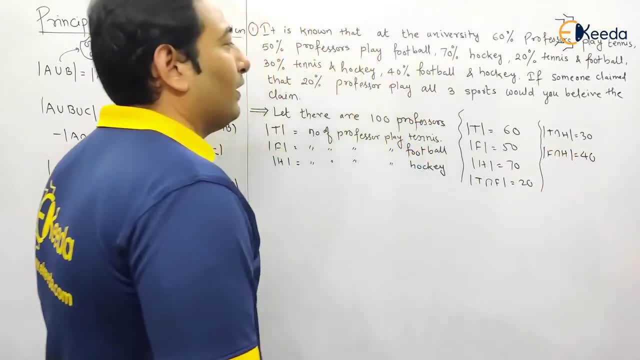 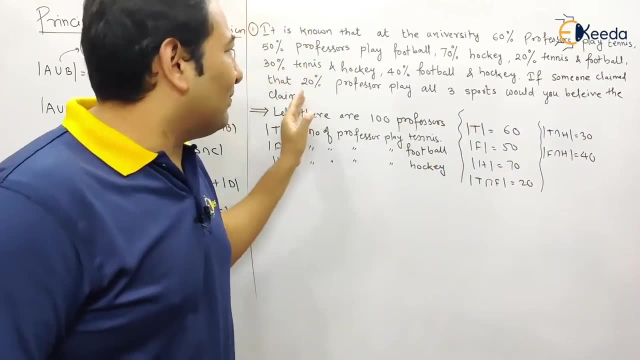 So football and hockey is 40%. If someone claimed that 20% professor play all the three sports, would you believe the claim? So this is what we going to check. So this is not given actually that we need to check it. 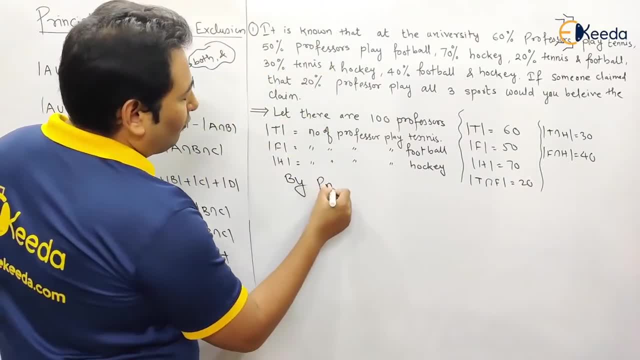 So let us start by Tennis and hockey: 40% football, 30% tennis and hockey. But this is for football, for hockey, to check whether this 20% is right or wrong. So this is not the data given. We need to find it. 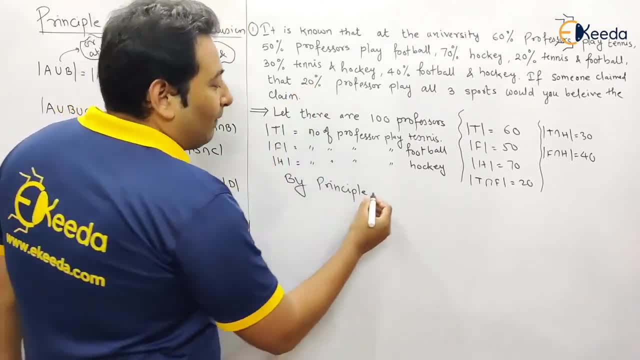 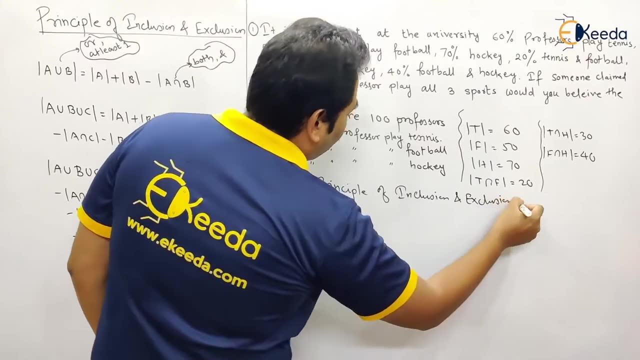 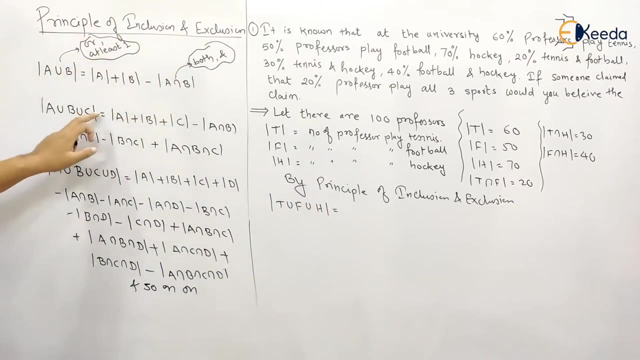 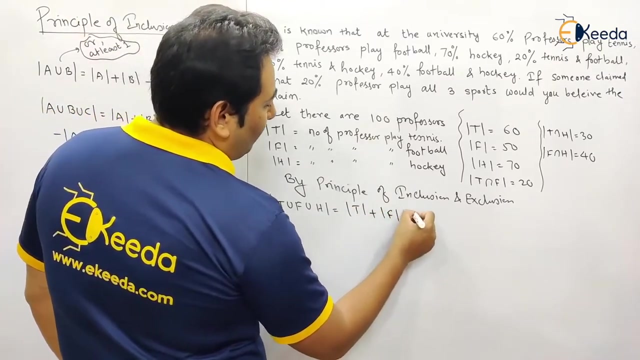 out the result and we need to verify whether it is right or wrong. By principle of inclusion and exclusion: T, union F, union H: See, this is the formula equivalent to this. All the single terms will be included. So T, F, H, All the double terms excluded. So what are the double terms? 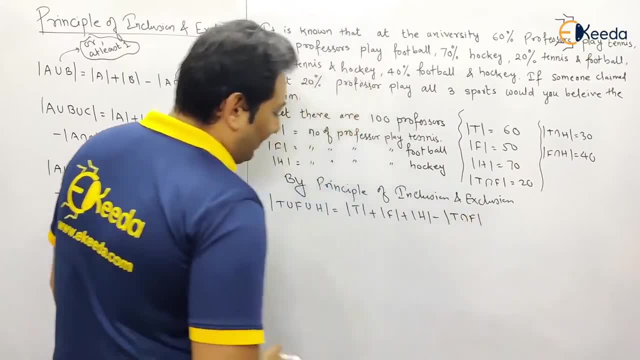 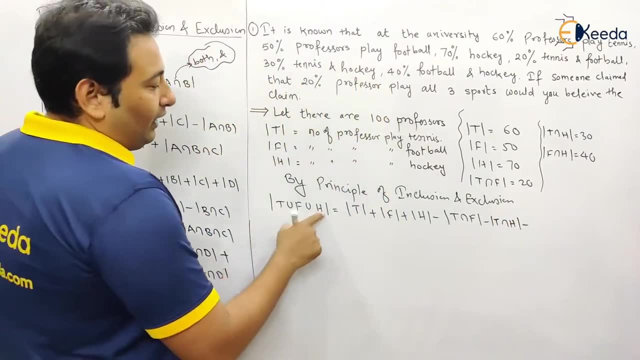 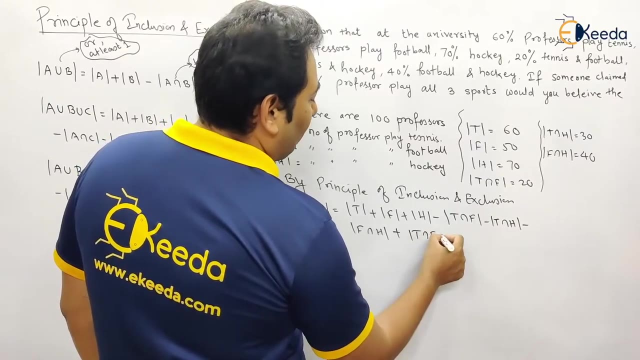 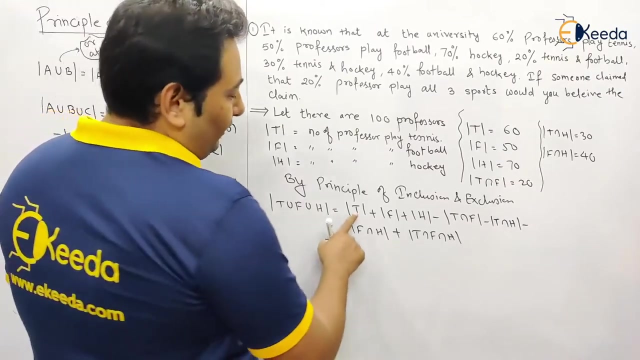 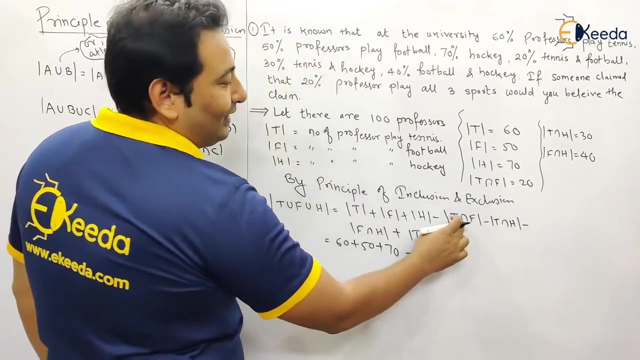 T and F. What next? T and H? Next F and H, Triple term will be included, That is, T and F and H. So which is equal to- let us fill the data here: t is 60 plus 50 plus 70 minus t and f, so t and f is 20. 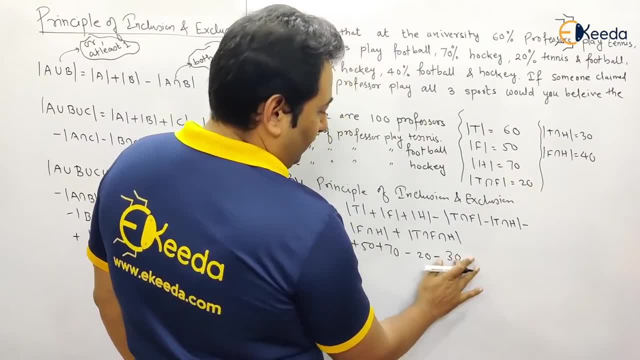 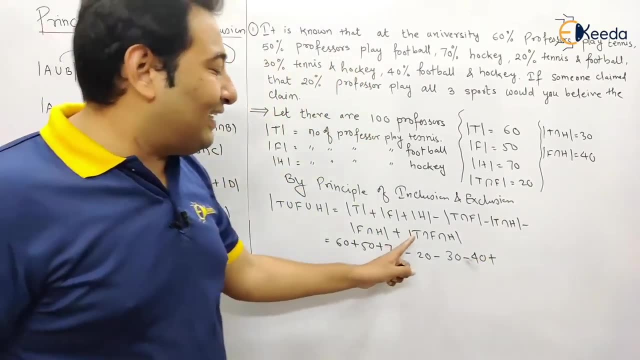 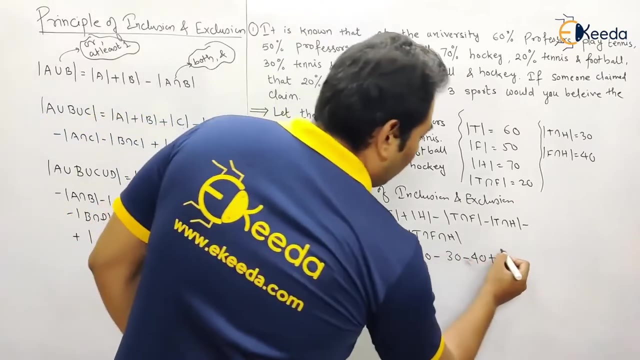 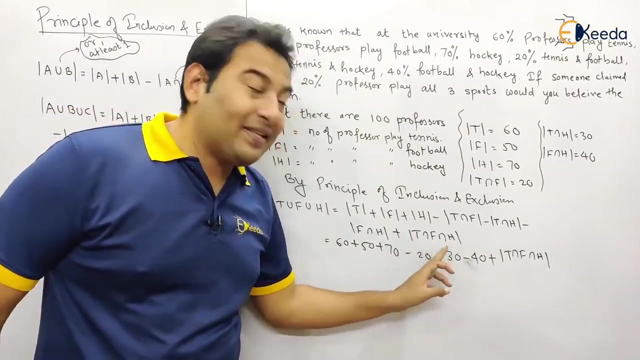 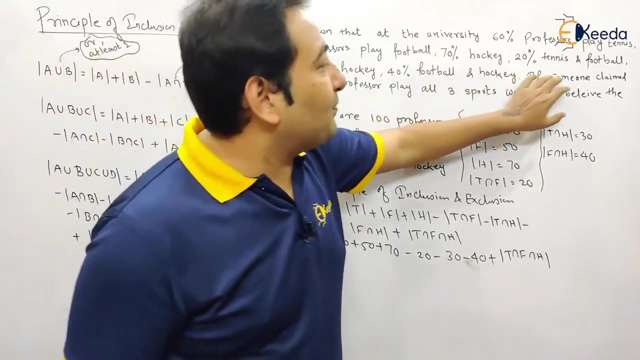 t and h is 30. uh, then f and h is 40 plus t and f and h. this is not known to us. what does this term mean? this term means professors play all the games and means all so professor that played tennis, football and hockey. this is not given see here. if someone claimed that 20 is their claim, that is not the answer. 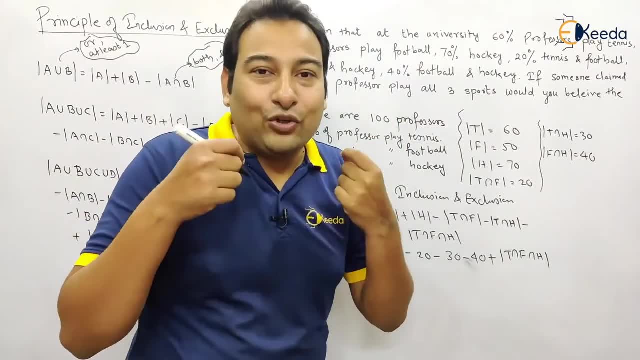 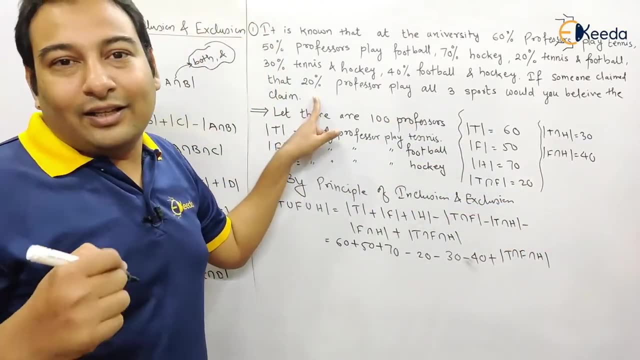 we need to find it out the value of this term and we need to check whether the claim is right or wrong. suppose this answer: if we get it as 20, then we'll say yes, 20 claim is right actually in this problem. we just need to find it out this term. 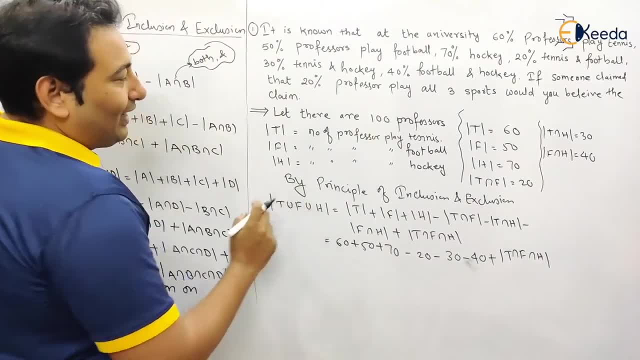 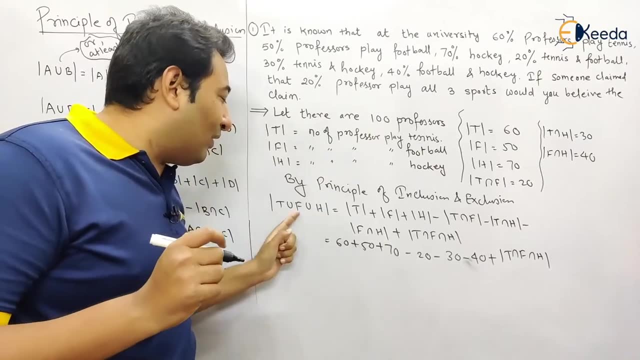 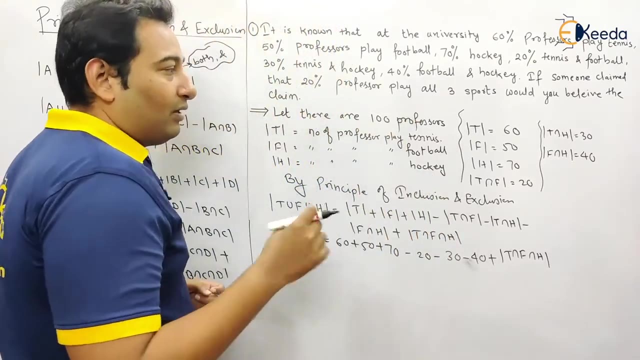 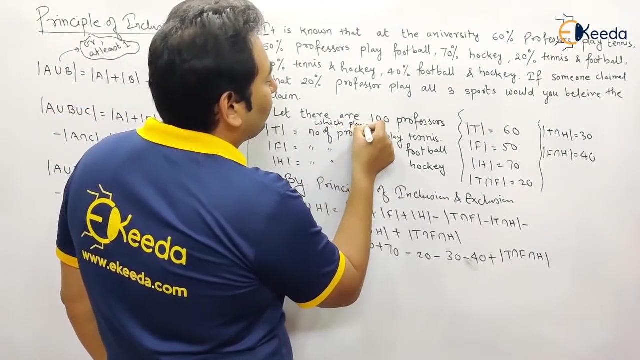 and what about this? is it given t, union f, union h? that means professor which play at least one game. this is the meaning, at least one. now here we assume there are hundred professors. it has to be a specific uh assumption: there are hundred professors which plays at least one game. if this is the assumption, then we can say: this value is hundred. see, there is a. 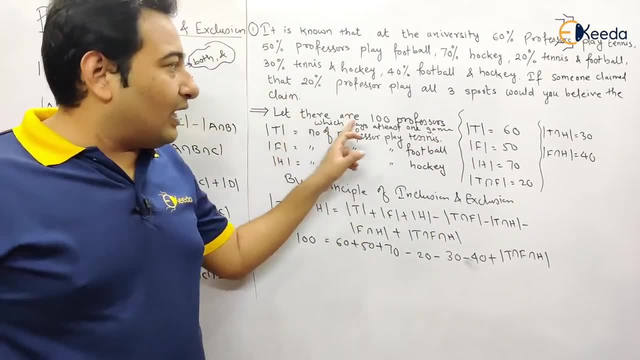 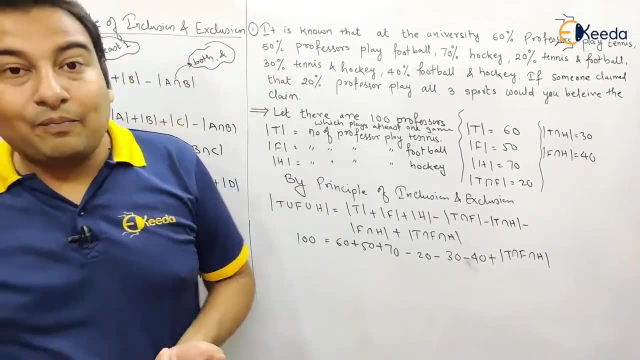 difference. there are hundred professors and there are hundred professors which plays at least one game. there is a difference because there might be a case there is, there will be a professor which does not play any of the game. so if you just assume, listen to me very carefully. if you just 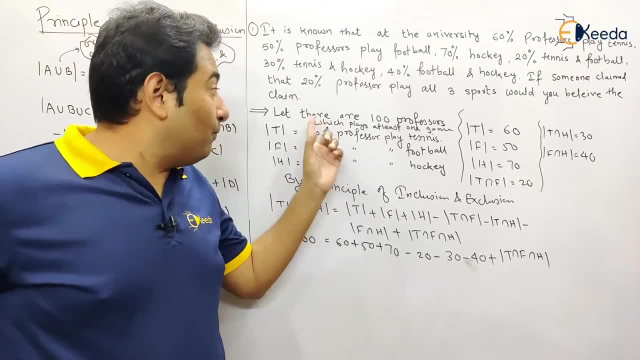 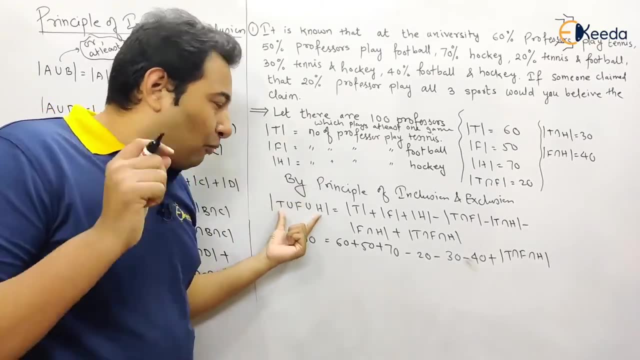 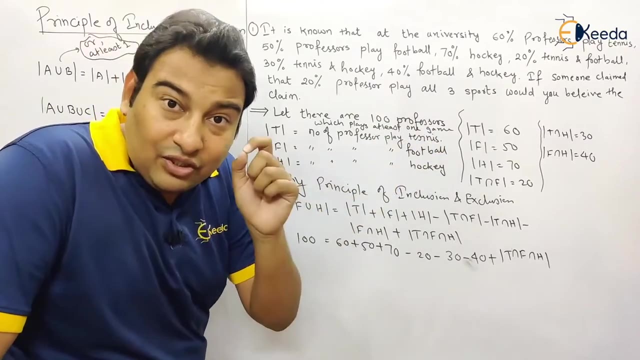 assume there are hundred professors. which does not play a game here, you cannot match their assumptions. in any case, professors, you cannot write it down here: hundred. what does this mean? this mean professor which plays at least one of the games. so if there are only hundred professor, there are hundred professor. if this is your assumption, you cannot write.